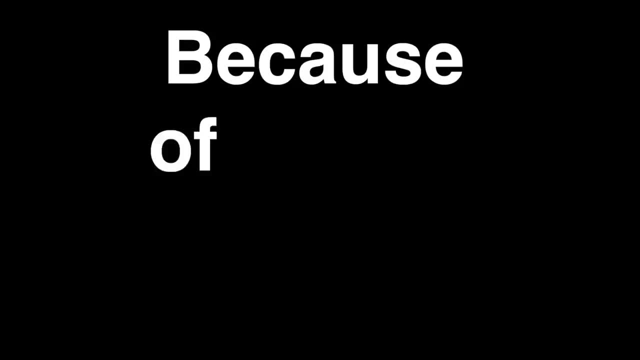 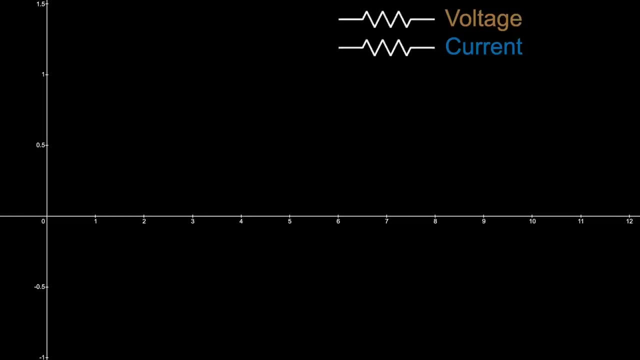 This video is sponsored by Brilliant. Because of phase and Euler's formula. These two things are pretty much the why and how electrical engineers use imaginary numbers in circuit analysis. With just resistors we don't need imaginary numbers because the ratio of voltage and current for a resistor is always constant. 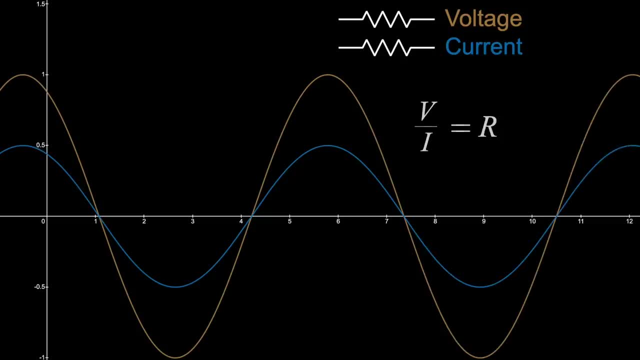 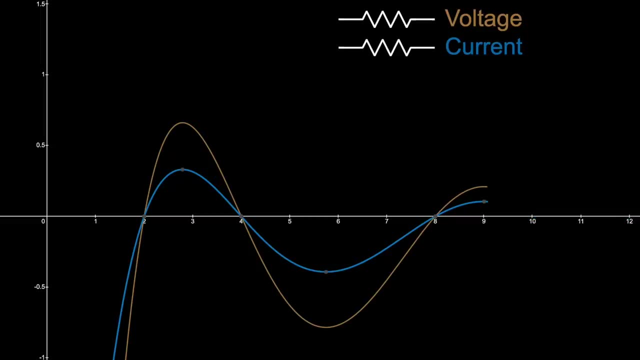 Thus they are in phase and the math is much easier. Even if the input is not sinusoidal, voltage and current will still move together With a capacitor. this is not the case If you have a sinusoidal input and plot voltage versus current across a capacitor. 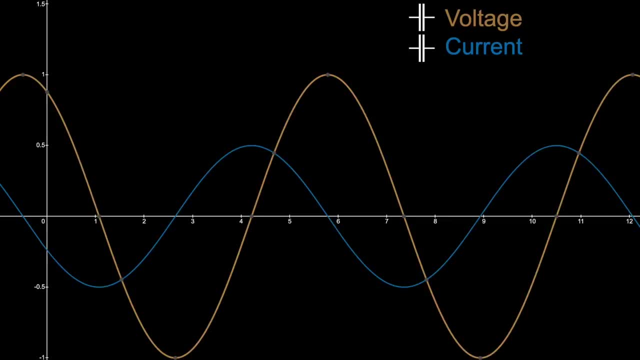 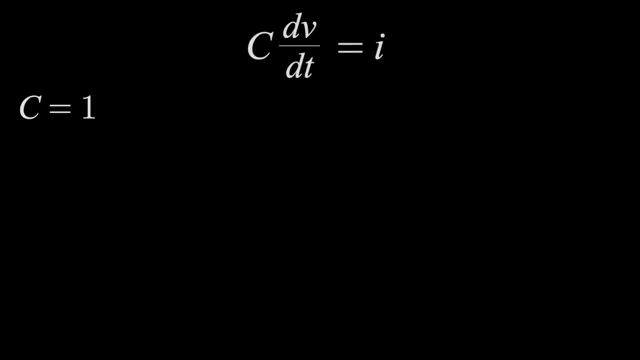 you'll find they are out of phase by 90 degrees, And that's found with the capacitor equation. So if I set C to 1, just for simplicity- and the voltage across the capacitor is sine t, then current is cosine t, which can also be written as: 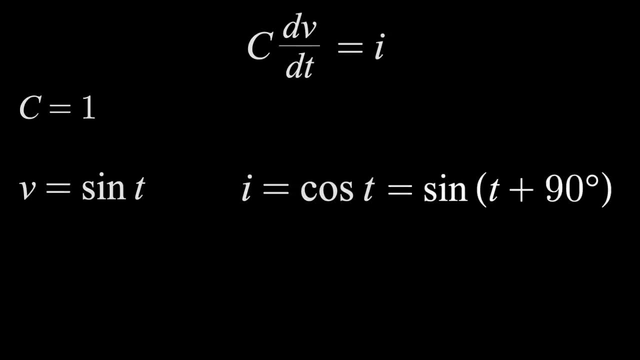 sine of t times sine of t. So, when it comes to sinusoidal inputs, capacitors cause this shift, along with likely an amplitude change. but the shift is what we care about, Because the math becomes more difficult when you have sinusoids with different phases. 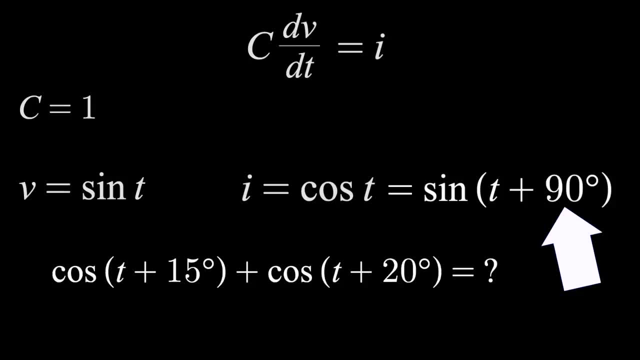 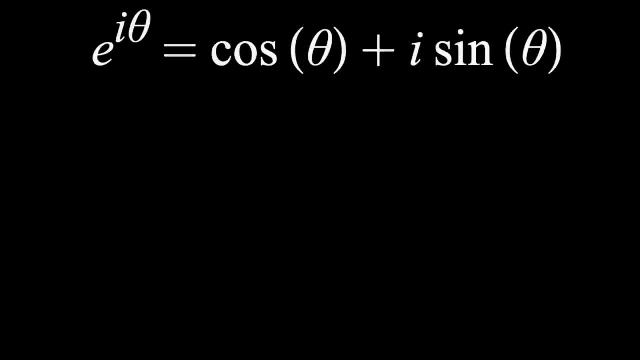 Even just adding. You can't just combine like terms here. You can use a trig, identity or something cooler, which is Euler's formula, and imaginary numbers. Now, the first reason that we're going to talk about sinusoidal inputs is that they are not just 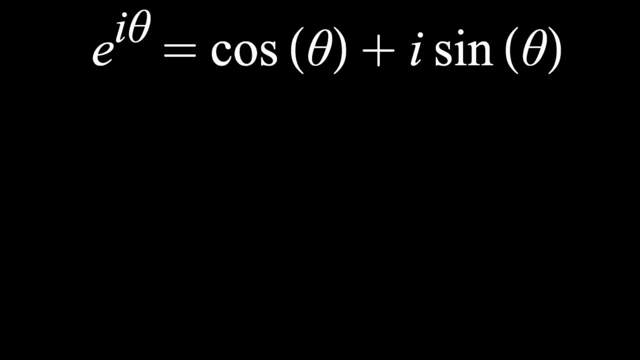 a formula. They are a formula that can be used to write any complex number in exponential form. I'm not going to go into the visuals of this, but as a numerical example, if you take the complex number 1 plus 1i, you can write that as root 2 cosine of 45 degrees. 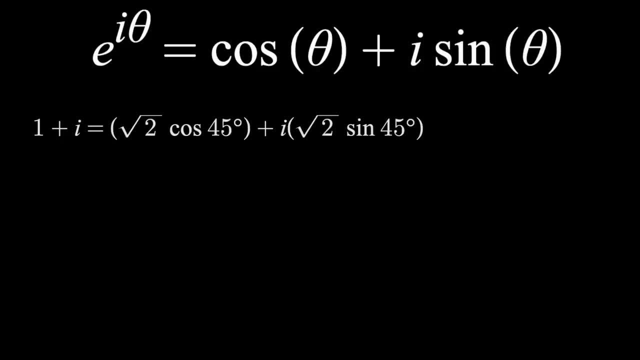 plus i times root 2 sine of 45 degrees, And this can be rewritten in exponential form according to Euler's formula. And all that matters here is the fact that this formula can be used to write any complex number in exponential form And this can be rewritten in exponential form according to Euler's formula. 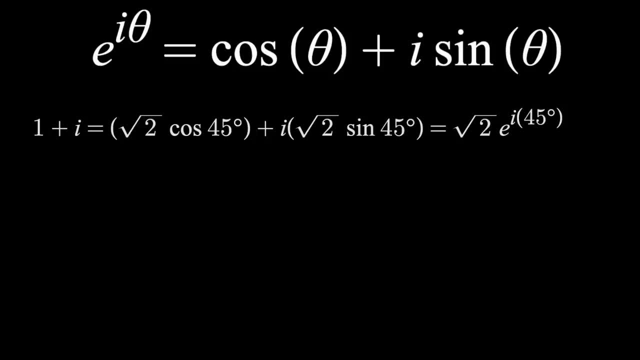 And all that matters here is the fact that this formula can be used to write any complex number in exponential form. The final point here is the fact that there's always a way to write a complex number in this format, which can then be rewritten in exponential form. 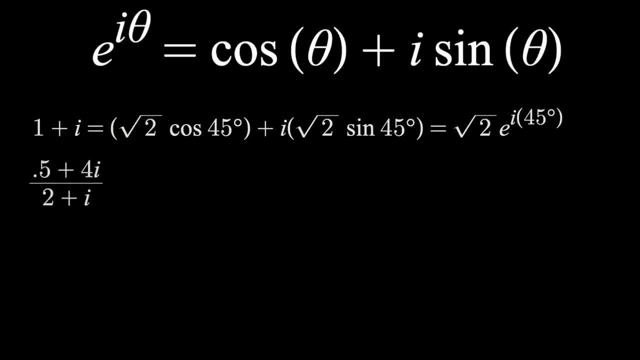 Even if that complex number looks like this, it can still be simplified to sum a plus b, i. Then, with just some basic trig, we find the real component 1 equals root 3.25 cosine of 56.3 degrees, while the imaginary component equals root 3.25 cosine of 55.3 degrees. which is exactly the same as the real component 1, we find, in this case, the real component 1 equals root 3.25 cosine of 56.3 degrees, While the imaginary component equals root 3.25 sine of 56.3 degrees. 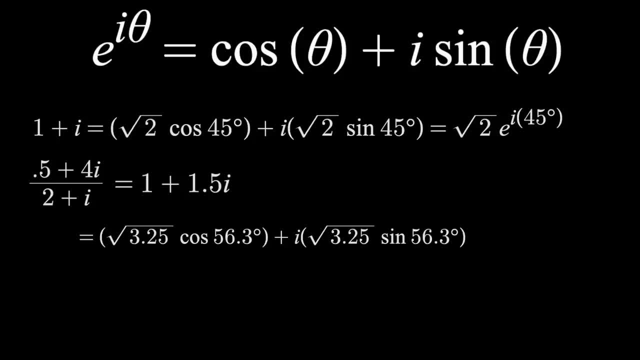 And now that we have the correct format, same coefficient and same argument, we can write this in exponential form. This is useful because when given a sinusoid there's no real constant. you can multiply it by to change the phase A. here only changes the amplitude. 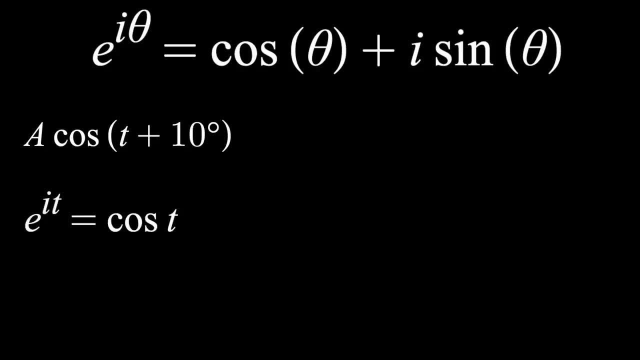 But if you have e to the i t which can be written out with sinusoids, and then multiply it by some complex constant, let's say 2e to the i times 30 degrees, which is just this. however, I'm going to keep it in exponential form, because all we have to do is use simple. 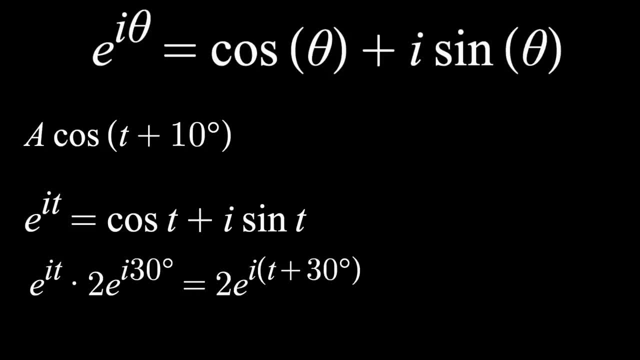 rules of exponents to get our answer Then from Euler's formula. we can write it out as such, And I know there are two sinusoids here. but just look at the individual components. Like the real part started out as cosine t. 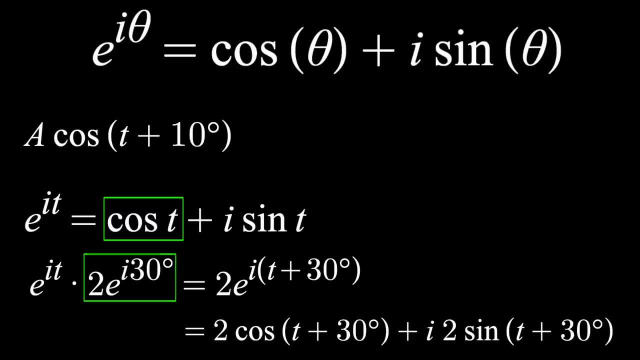 After multiplying by sinusoids, we get sinusoids, So we can write it out as sinusoids By just a complex number. the real part of the output is still just a cosine function, but with a different amplitude and phase, which is exactly what we observe with voltage. 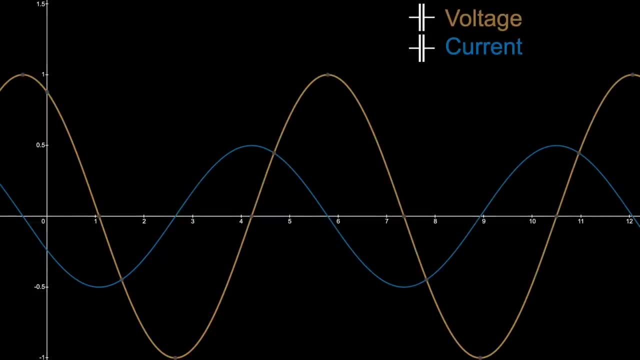 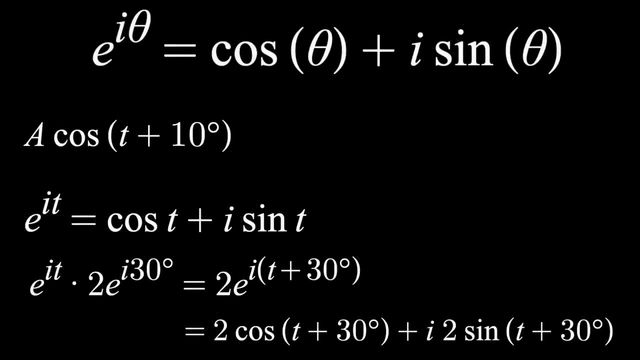 versus current in a capacitor or inductor. So there's a peek at how useful complex numbers are. They help when amplitude and phase shifts occur. Now, another thing we can do with Euler's formula is essentially solve problems that involve sinusoids by replacing them with this exponential. going through with the math. 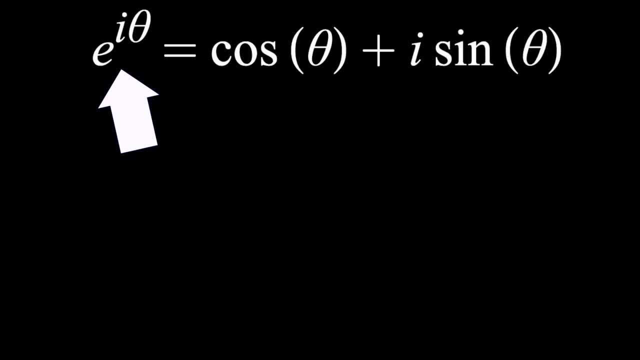 then just looking at the real component of the output. Not a great explanation, but here's what I mean. You can find the double angle formula for cosine, as well as many other trig identities, by just using Euler's formula. The first step is to just plug 2theta into the argument, because now the real part of 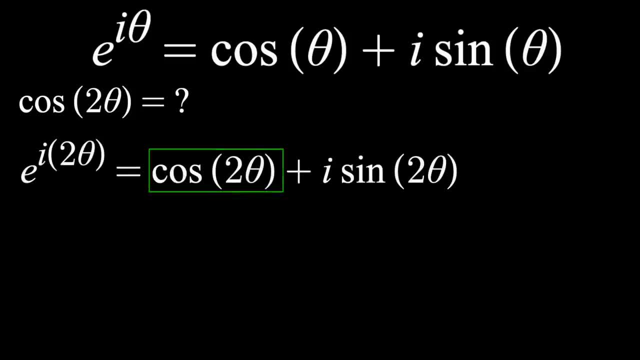 this is what we're trying to find a formula for, And now you can use a simple rule of exponents to rewrite the left side as e to the i theta all squared, which is just Euler's formula squared. If we foil this out using the fact that i squared is negative 1,, we'll get this here. 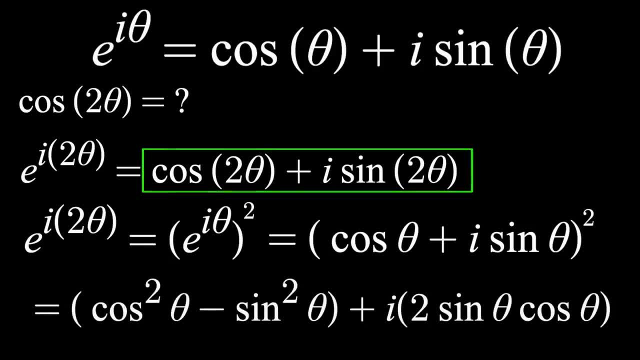 which again is equal to what we started with e, to the i times 2 theta. So setting the real parts equal to one another, we get cosine of 2 theta equals cosine squared minus sine squared, which, hey, is the double angle formula for cosine. 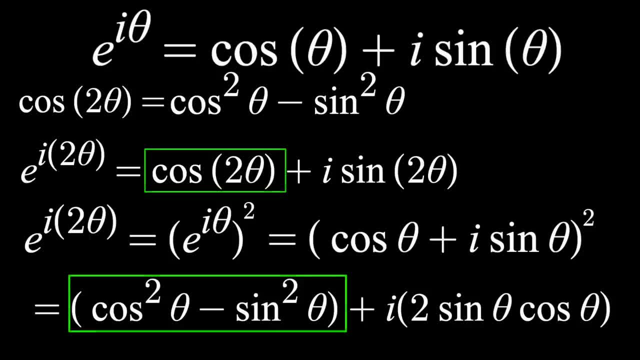 But that's not all, as the double angle formula for sine can be found by setting the imaginary components equal to one another. So that's the idea. When given a problem with cosine of something or sine, sometimes, we can instead make it more complicated by adding i sine of that thing and setting it equal to our exponential. 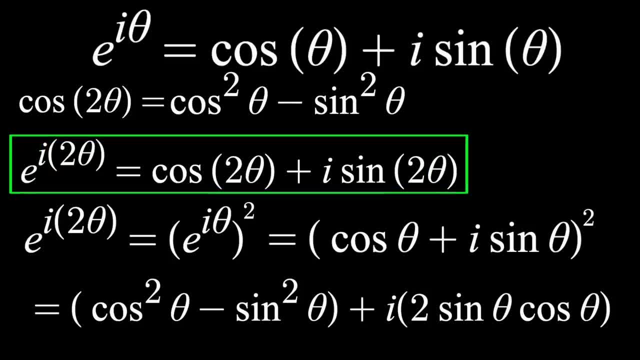 Because now we can use properties, Properties of exponents to simplify this And, at the end, the individual components in a way reveal our answer. By the way, that's also how you can solve this problem. I put on the screen earlier. 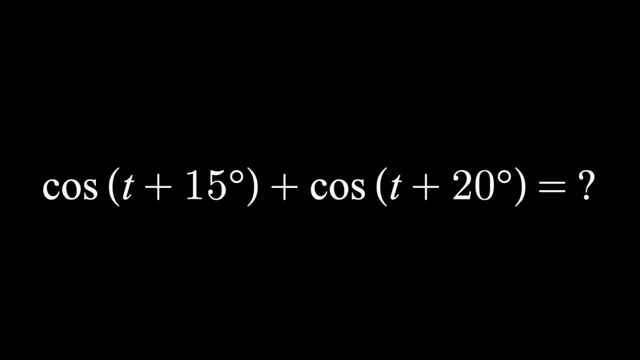 Just put them in exponential form, simplify, then look at the real component. So now let's apply this to the capacitor equation And because i is used for current, to avoid confusion from here on, the imaginary unit will be represented with a j instead of i. 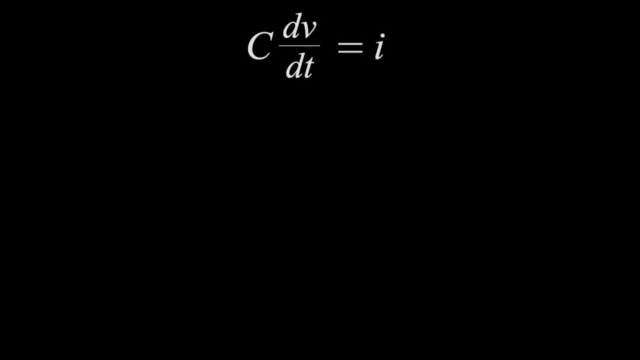 Which is actually what electrical components are, And that's what electrical engineers do. Now, if the input is a generic sinusoid, some a cosine of omega t plus theta, well, again we can find current by just taking a derivative. So we get current. is this here? 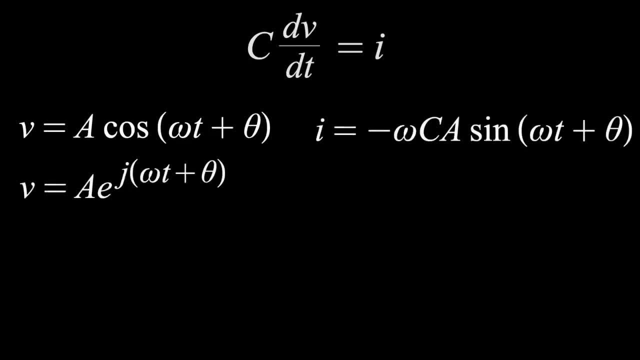 But let's instead say voltage is ae to the j times, omega t plus theta, Which is weird and makes no sense physically. but the real part of the exponential is our actual voltage. So at the end we'll just see what the real component looks like. 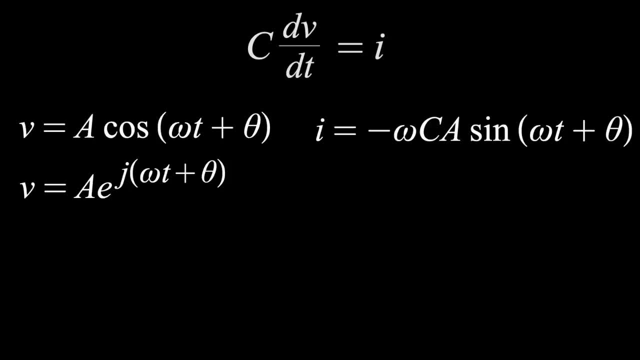 Ok, so we'll go through with the derivative and j root. negative one is just a constant, by the way. So we get current equals this here, But ae to the j omega t plus theta is just our voltage, So we can actually say current equals j omega c times v. 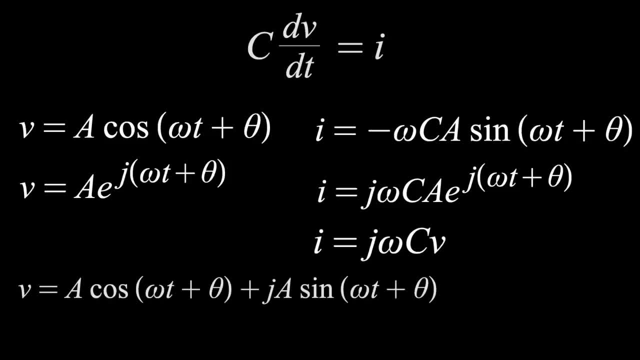 And voltage as we've defined it is this here with the real and imaginary components. So multiplying that by j, omega, c, we get this, And if we just look at the real component, we see it's the same as what we got before. 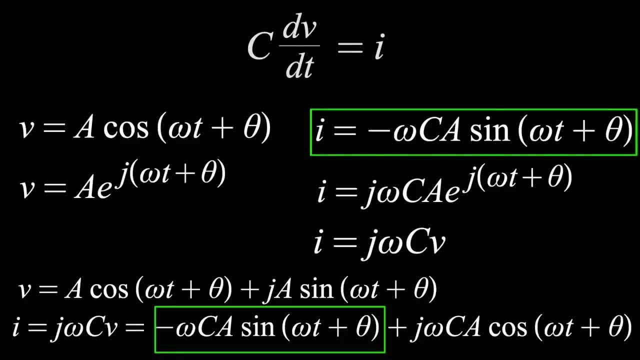 when we simply took a derivative of a cosine function. Now, Euler's formula did not make any of this any easier. But notice how, by using Euler's formula, we turned an equation that involves a derivative into one that doesn't. That's the key detail. 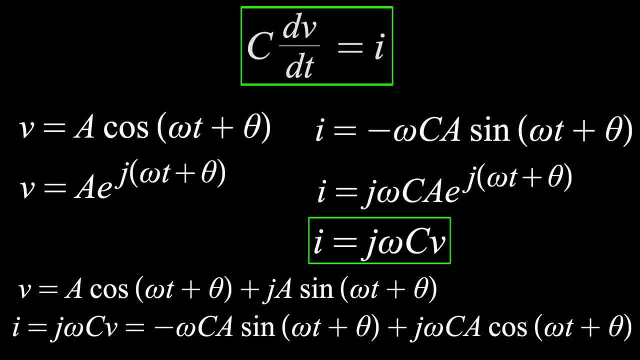 That makes this all useful for real circuits, Because now we can rearrange this equation and make a ratio of voltage and current. This is the impedance of a capacitor, which is kind of like resistance. The 1 over omega c part is the ratio in amplitude a versus omega c a. 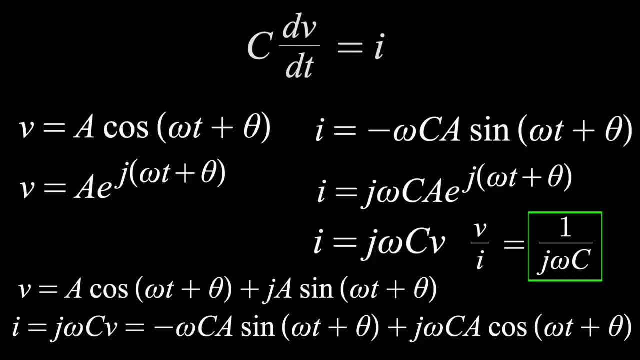 But the j, the imaginary unit, tells us there will also be a phase shift of 90 degrees Cosine versus negative sine. And this is what we get. So now let's put it all together with a circuit that has a resistor, a capacitor. 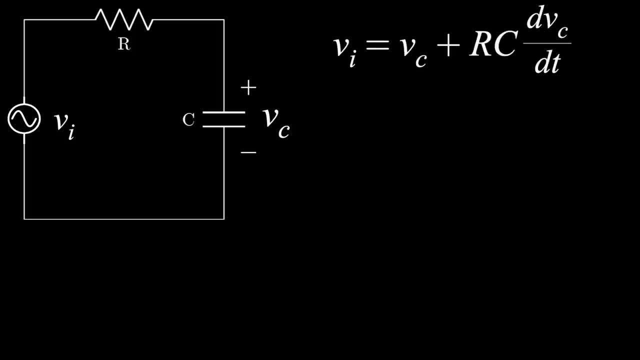 and a sinusoidal input. This is the actual differential equation that would be used to solve for the voltage across the capacitor. But if the input is sinusoidal, then the capacitor voltage will be as well. So we know the solution is going to have the form A cosine of omega t plus theta. 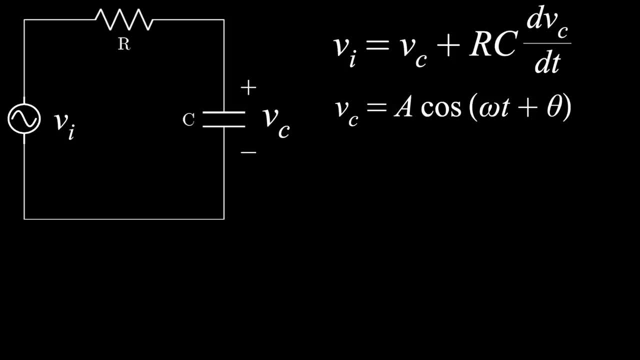 But instead of plugging that in for V sub c and solving, Which would not be fun, We can instead say: V sub c: is this exponential? Because, as we just saw, the time derivative of this is j, omega times itself, Vc. 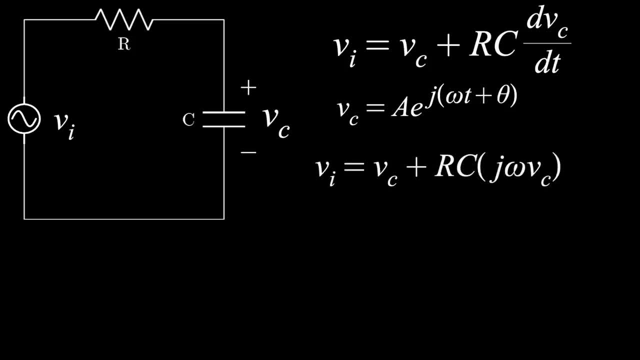 So plugging that in for dv, dt, the differential equation becomes an algebraic one, And after factoring out a V sub c, then rearranging the capacitor voltage we're looking for comes out to 1 over 1 plus j, omega times itself. 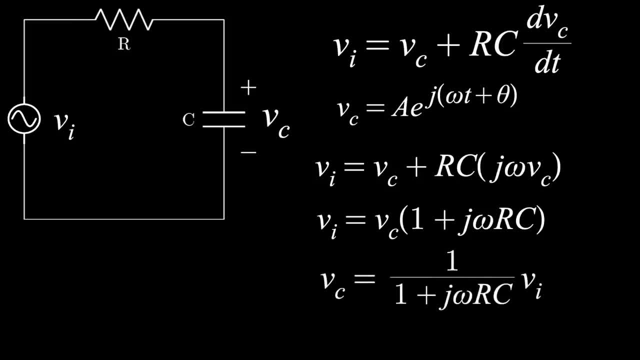 This is an algebraic equation, So we can just plug that in for dv, dt, j, omega, rc times the input voltage, And this is just a complex number which can be rewritten using Euler's formula. So I need to make some room here. 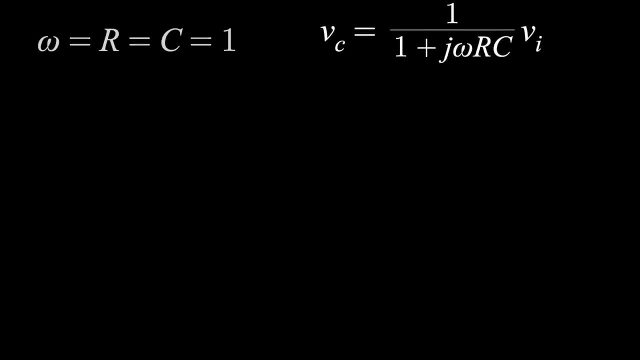 but if omega r and c are all, let's say one, then the coefficient becomes one over one plus j, which can be rewritten as 0.5 minus 0.5j, or root two over two times e to the j. 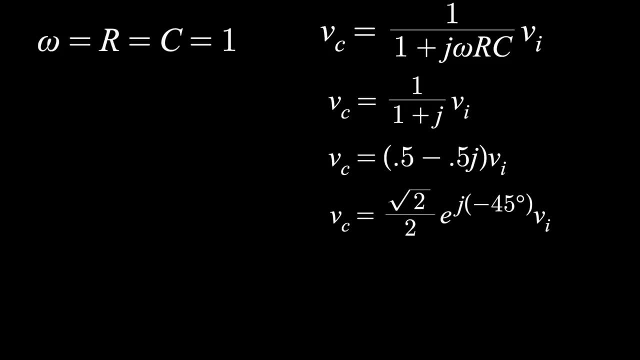 times minus 45 degrees. So if the input voltage is something like three cosine of t plus 10 degrees, we can replace that with Euler's formula or put it in phasor form, knowing the actual voltage is the real component. So if we plug that in for the input voltage, 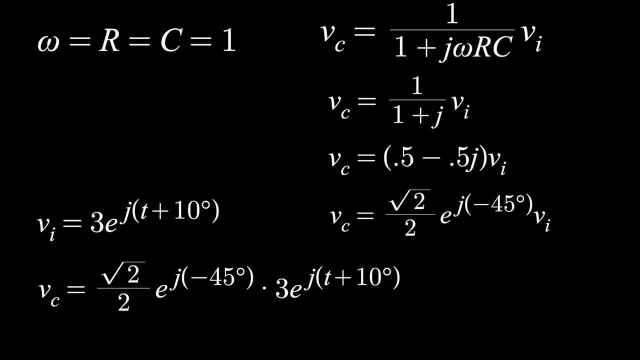 then we find the output voltage across the capacitor. is this here? But of course we only care about the real component, which is three root, two over two, cosine of t minus 35 degrees. That's how imaginary numbers help us, Instead of having to solve a differential equation. 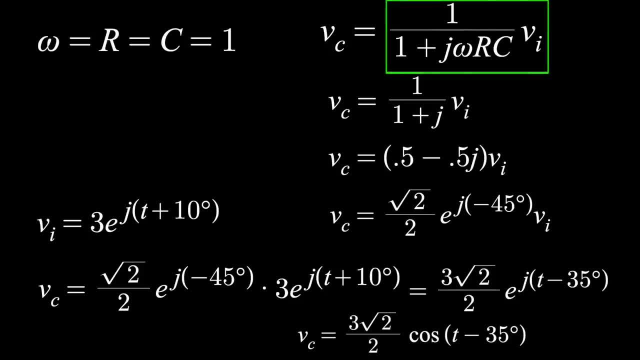 we can solve an algebraic one with imaginary numbers. Once we have this equation, the only math we have to do is figure out what that complex coefficient is in exponential form, Because that exponential tells us, in this case, that we have to multiply the input voltage, amplitude. 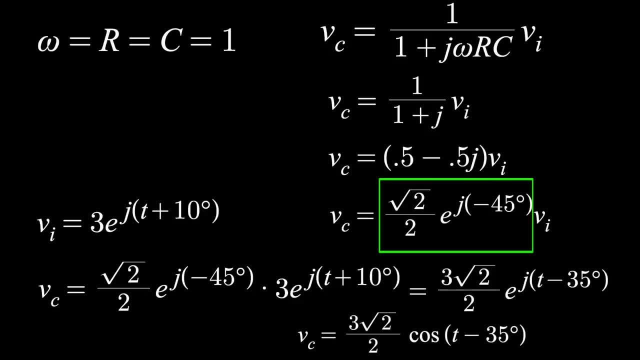 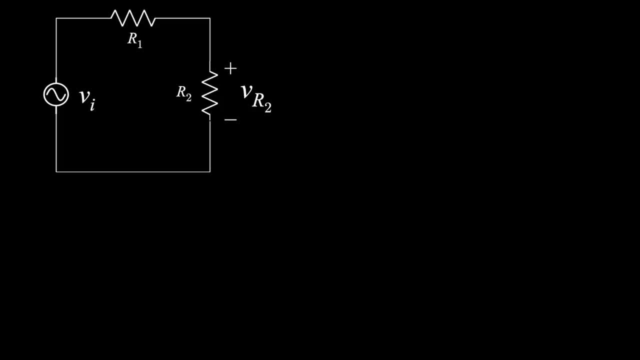 by root, two over two, and shift the phase by negative 45 degrees. And when you have a circuit with just resistors, to find the output voltage across R2, you use this equation, a simple voltage divider, When R2 is replaced by a capacitor. 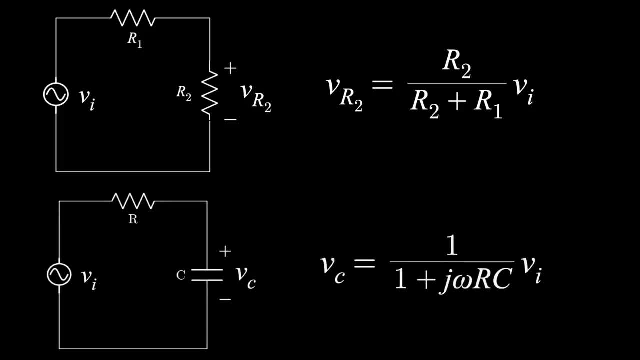 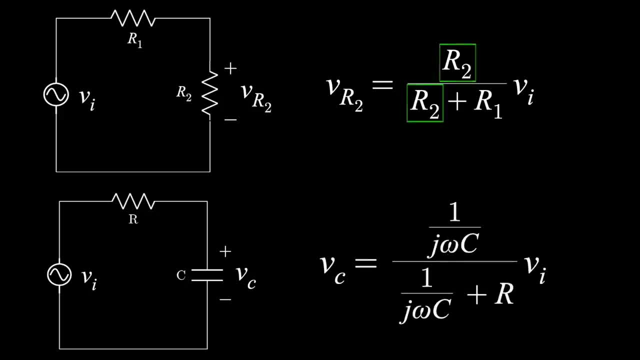 which hey looks very similar to the equation, which hey looks very similar to the equation above, Just instead of R2, we have one over j, omega c, which, remember, is the impedance of the capacitor. So we can treat impedance just like resistance. 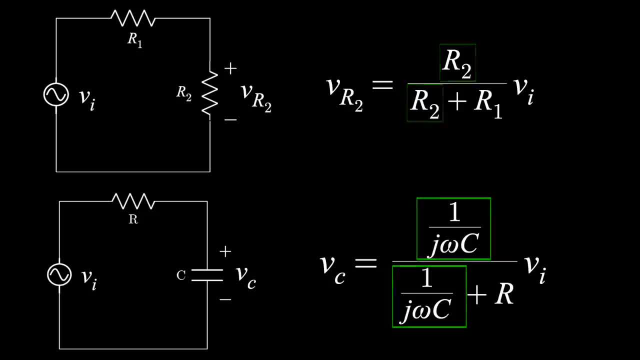 in that we can add the values when components are in series, we do the reciprocals when they're in parallel. but the only difference is you're gonna get complex numbers because there will be a phase shift- that happens as well as an amplitude change. 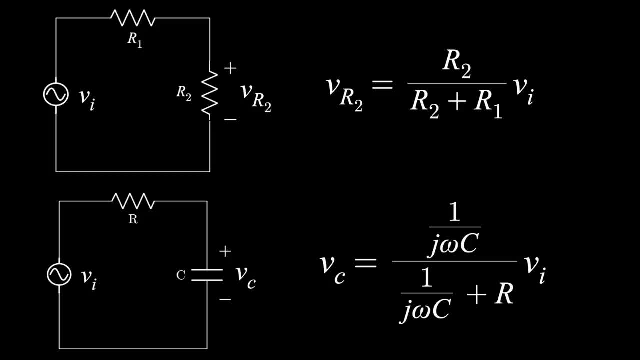 which we can find algebraically using Euler's formula. And while this is all useful for sinusoidal inputs, when you have anything else the math actually still works for the most part, because all functions can be made up of sinusoids. It's beyond this video. 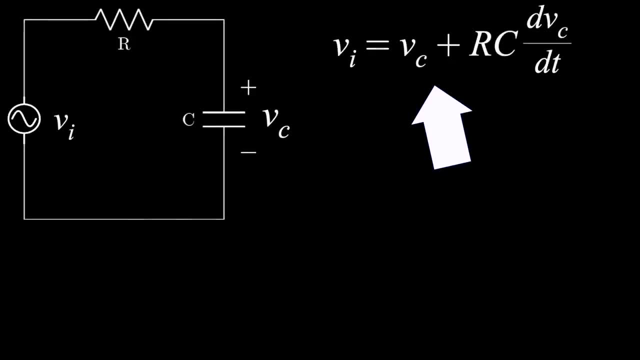 but if you apply the Fourier transform to both sides of this equation or the capacitor slash inductor equations, you get the same impedances and voltage dividers as before. You would just have to do inverse transform with the same number of terms at the end. 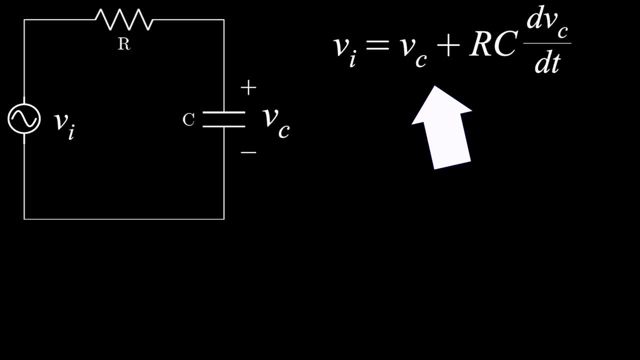 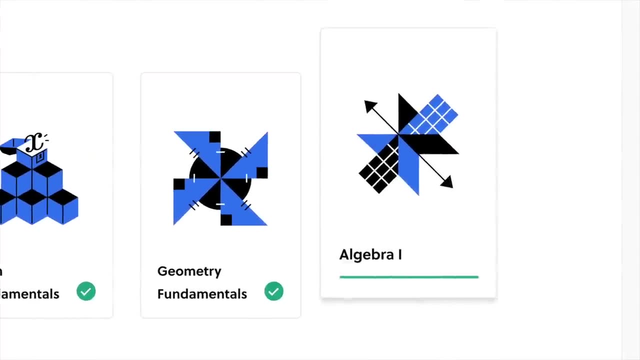 to get an actual solution, And if you wanna see more of the real-world applications of complex numbers, you can do so on Brilliant, the sponsor of this video. Brilliant is an educational platform home to thousands of lessons in math, science and engineering. 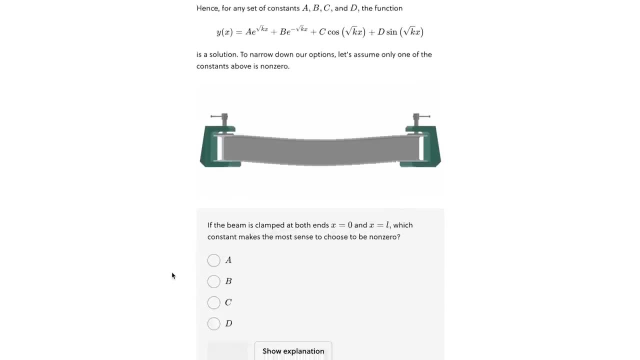 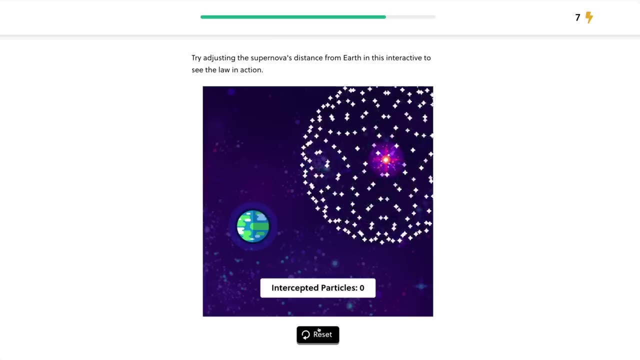 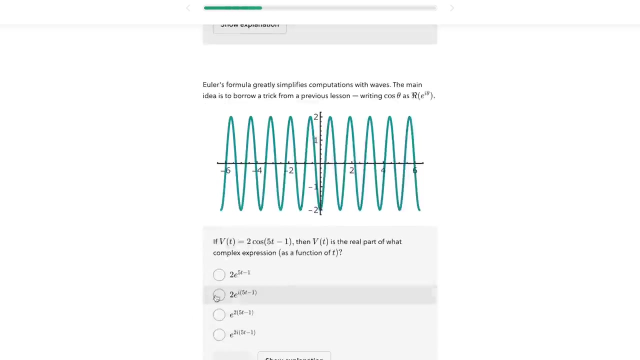 with new lessons being added monthly, And a big focus with Brilliant is real-world applications, as they show you exactly how to apply the formulas and concepts within their lessons. Here you can see some examples from their complex numbers course, which dives much deeper into the power of Euler's formula. 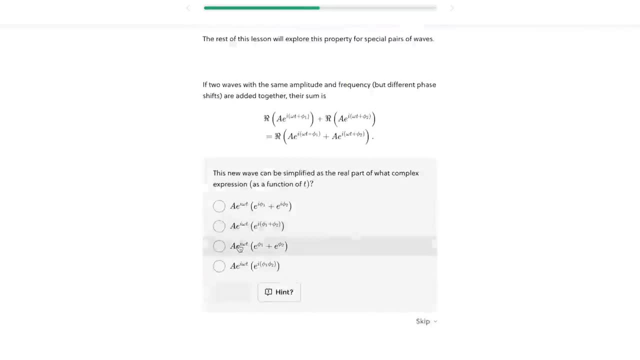 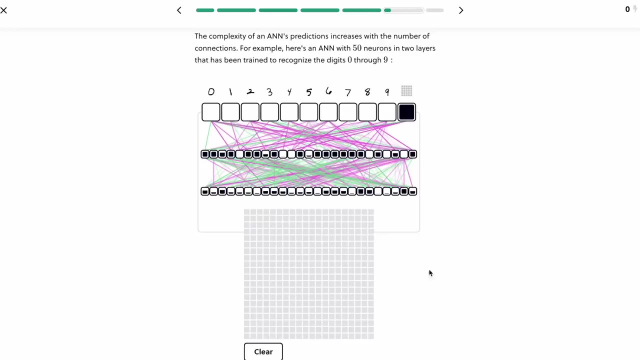 and what can be done with it. And, as with all their courses, you get constant practice problems, as well as intuitive visuals that help you understand even the more advanced concepts on a fundamental level, And you can now try everything Brilliant has to offer. 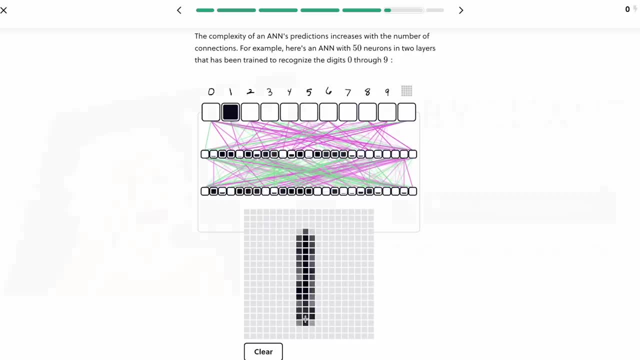 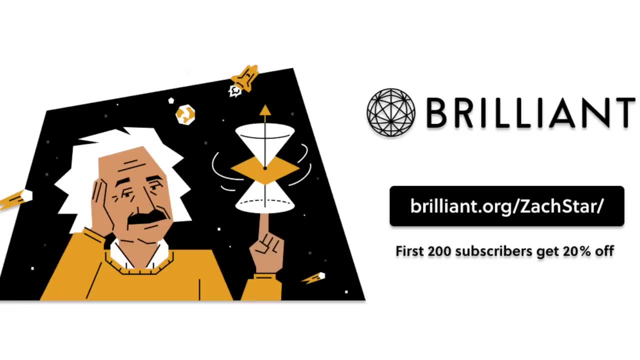 free for a full 30 days. Just go to brilliantorg, slash Zach Starr or click the link in the description below. plus, the first 200 of you to sign up will get 20% off Brilliant's annual premium subscription. With that gonna end that video there. 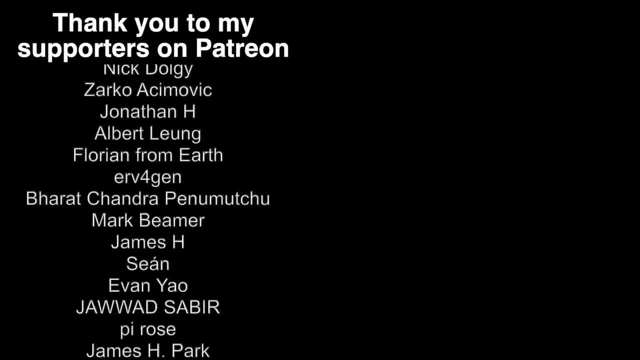 Thanks, as always, to my supporters on Patreon. social media links to follow me are down below and I'll see you all in the next video.